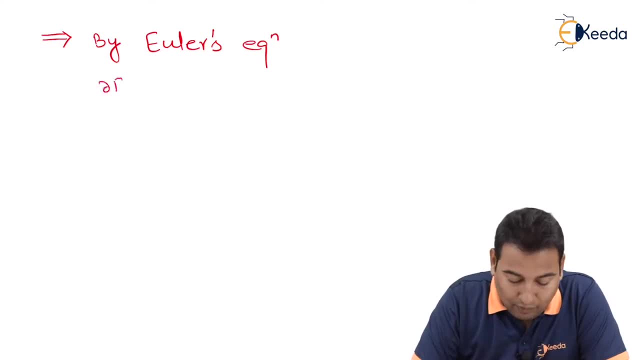 By Euler's equation. we have two options. The first is dof upon do y minus dy. by dx of dof upon do y, dash is equal to zero. This is the first equation. If you observe the problem, functional is independent of y. What does that mean? Dof upon 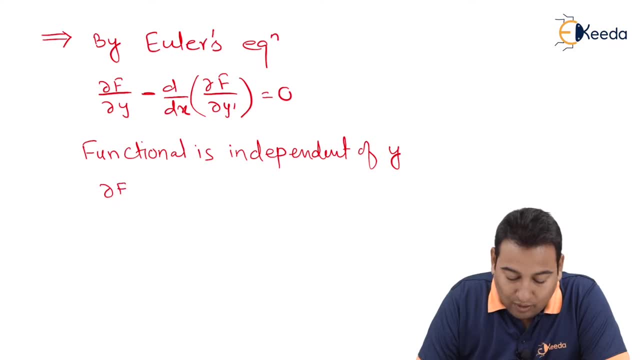 z is equal to zero. If you observe the problem, functional is independent of y 這邊이번. Olá 당신 taxi제i 계�. станов음 dof 위는 코 wra 45.. y 값 conveyed도 questions Mehr Krankenām. 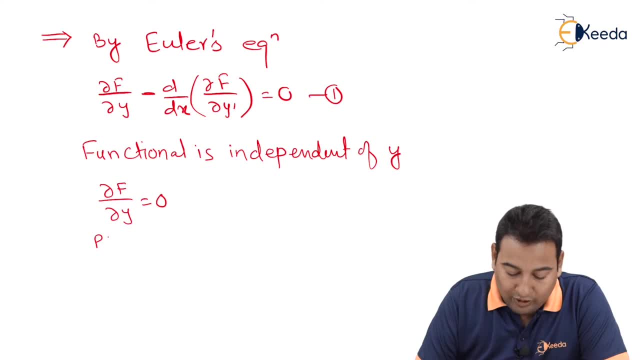 다른 말로 뜻: proteins. estou 업çon 잠깐 방문ml. 0 put in 1. if you substitute in equation number 1, this will be 0. you will be left with minus d by dx of dou f upon dou y dash equal to 0. if this minus d by dx will go that side and that will. 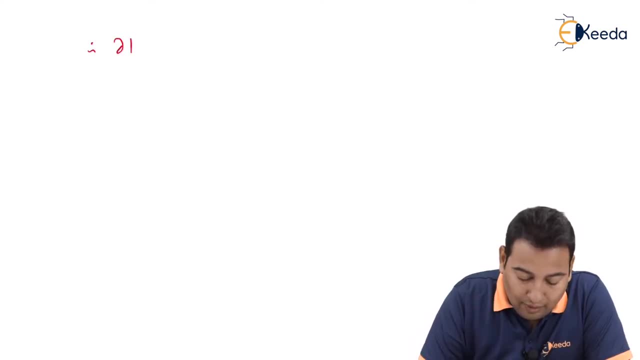 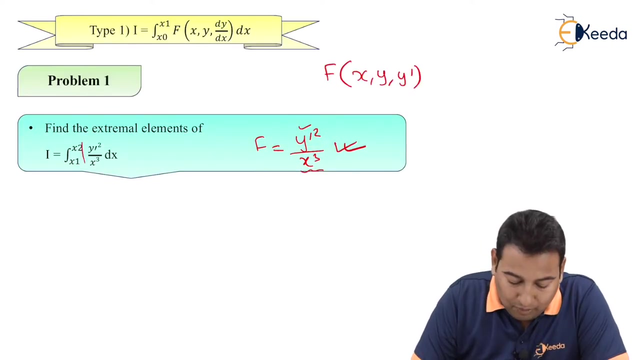 become c. therefore, dou, f upon dou, y dash equal to c. this we have already discussed in first video. this is just a revision part. let's move on and let's check what is f given in the problem. f given in the problem is this: that is, y dash square upon x cube. therefore, this will be dou upon dou. 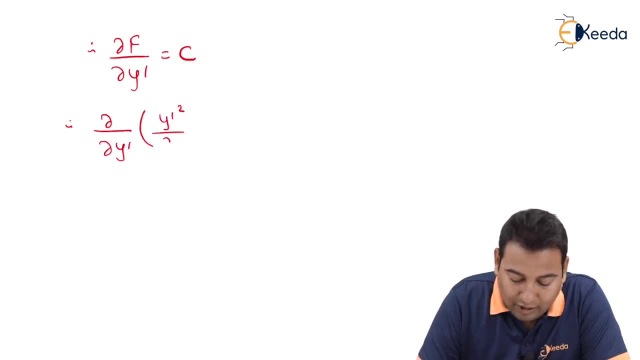 y dash of f, that is, y dash square upon x cube equal to c. we need to solve this to get the solution. as this is discussed, the solution will be in terms of y is equal to fx. this will be the required solution. basically, i want y, that's it. 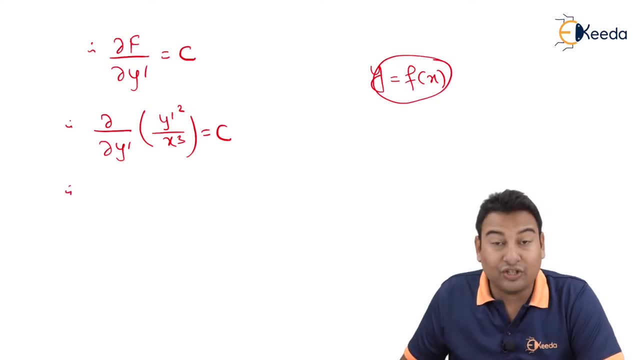 let's differentiate- this is your partial differentiation- dou upon dou: y dash with respect to y dash, x and y constant. functional is in terms of x, y and y dash. if you differentiate with respect to x, y, y dash constant. if you differentiate with respect to y, x, y dash. 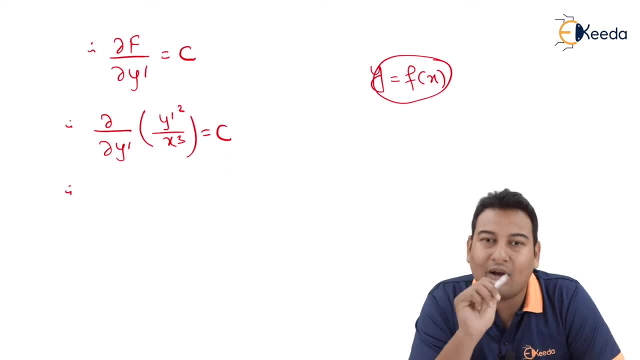 constant. if you differentiate with respect to y dash, x and y constant, here, friends, we are constant, x and y. therefore one upon x cube is constant. will come out: y dash. square derivative with respect to y dash is 2y dash. same way, x square derivative with respect to x is 2x.